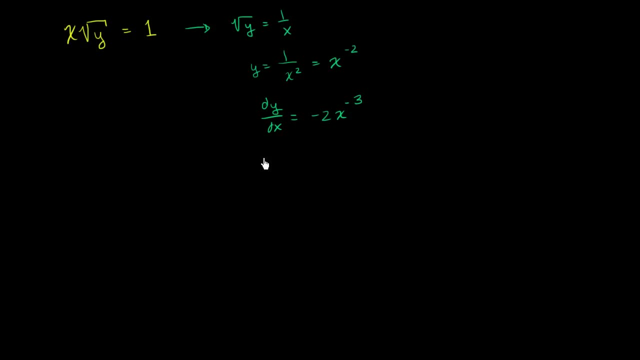 to the negative 2 minus 1, x to the negative 3 power. So that's pretty straightforward. But what I want to see is if we get the same exact result when we differentiate implicitly. So let's apply our derivative operator to both sides of this equation. 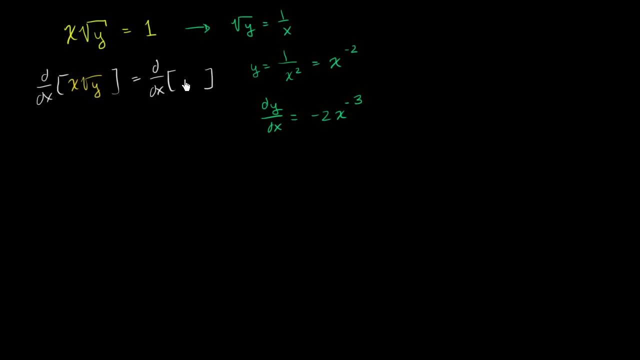 And so let me make it clear what we're doing: x times the square root of y and 1 right over there When you apply the derivative operator to the expression on the left-hand side, we are just going to have to apply both the product. 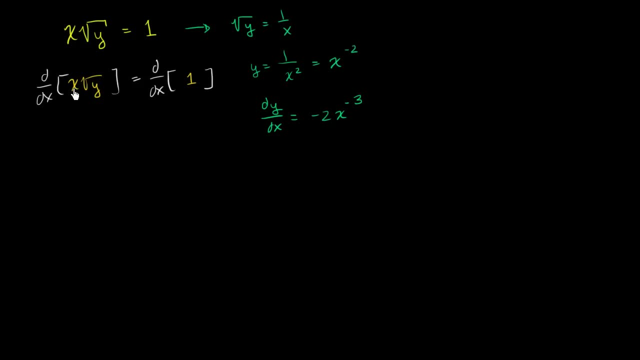 rule and the chain rule. The product rule is the chain rule. The product rule tells us: so we have the product of two functions of x. You could view it that way. So the product rule tells us this is going to be the derivative, with respect, 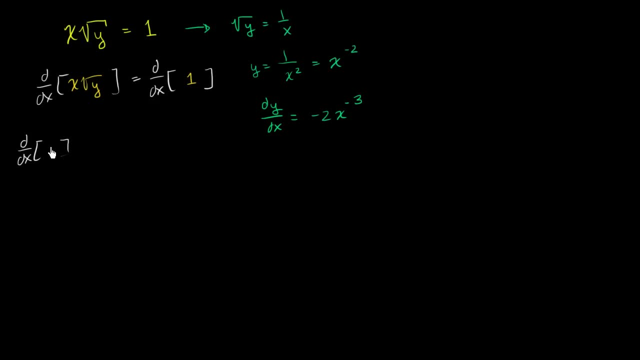 to x of x times the square root of y plus x, not taking its derivative. plus x times the derivative with respect to x times the derivative with respect to x of the square root of y. Let me make it clear this bracket Of the square root of y. 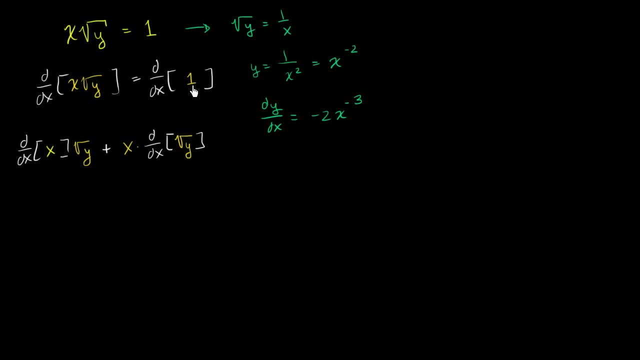 And on the right-hand side, right over here, the derivative with respect to x of this constant, that's just going to be equal to 0.. So what does this simplify? to Well, the derivative with respect to x of x is just 1.. 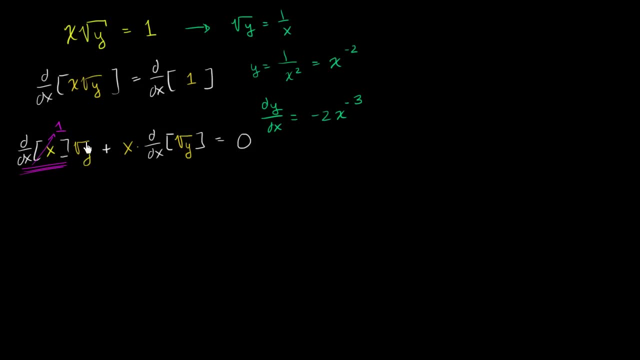 This simplifies to 1.. So we're just going to be left with the square root of y right over here. So we're just going to be. this is going to simplify to a square root of y. And what does this over here simplify to? 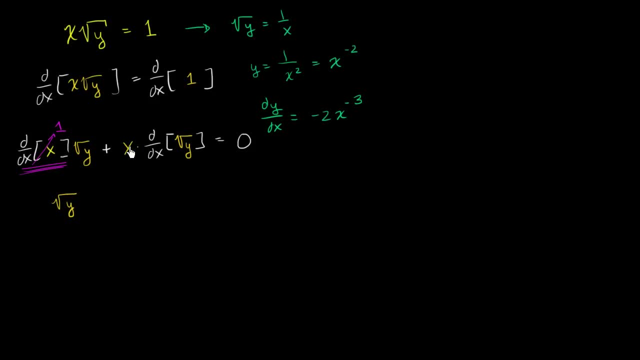 Well, the derivative, with respect to x, of the square root of y. here we want to apply the chain rule. So let me make it clear. So we have plus this x, plus this x, plus whatever business this is, And I'm going to do this in blue. 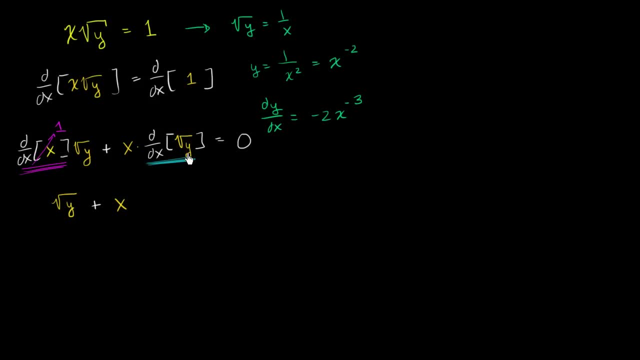 Well, it's going to be the derivative of the square root of something with respect to that something. Well, the derivative of the square root of something with respect to that something, or the derivative of something to the 1 half with respect to that something. 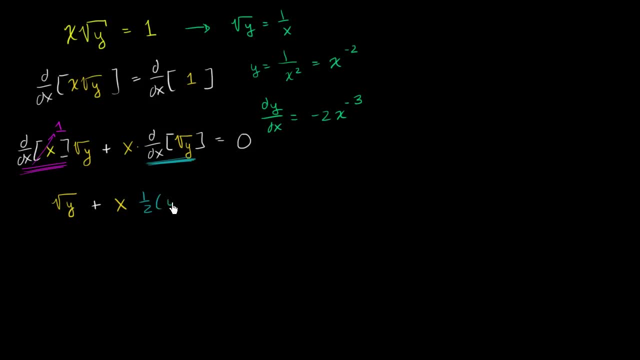 is going to be 1 half times that, something to the negative 1 half power. Once again. this right over here is the derivative of the square root of y with respect to y. We've seen this multiple times. If I were to say the derivative of the square root. 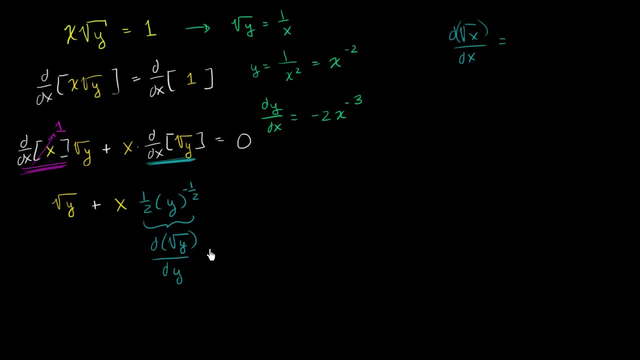 of x with respect to x, you would get 1 half. x to the negative 1 half. Now I'm just doing it with y's, But we're not done yet. Remember our derivative operator wasn't to say with respect to y. 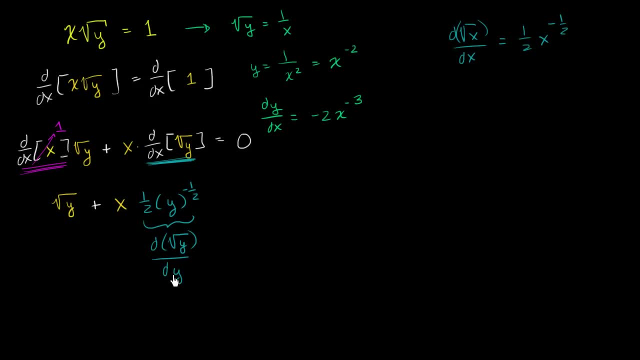 It's with respect to x, So this only gets us with respect to y. We need to apply the entire chain rule. We have to multiply that times the derivative of y with respect to x in order to get the real derivative of this expression. 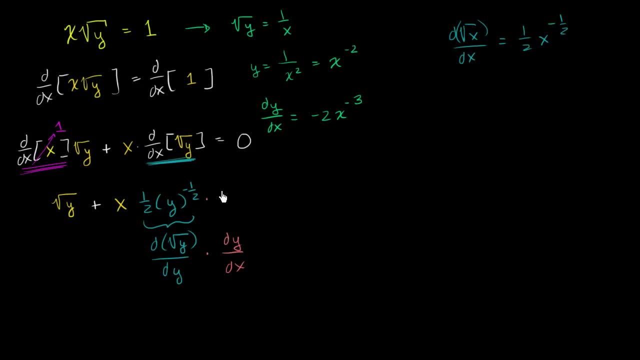 Absenteeism with respect to x. So let's multiply times the derivative of y with respect to x. We don't know what that is. That's actually what we're trying to solve for, But to use the chain rule, we just 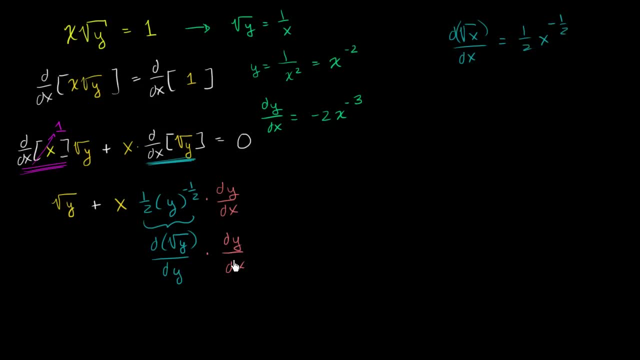 have to say. it's the derivative of the square root of y with respect to y times the derivative of y with respect to x. This is the derivative of this thing with respect to x. So we get this on the left-hand side. On the right-hand side we just have a 0.. 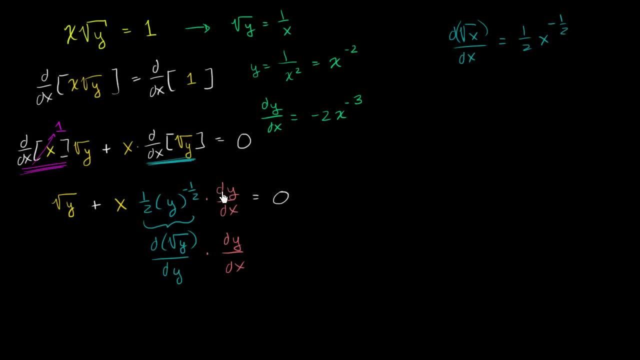 And now, once again, we can attempt to solve for the derivative of y with respect to x, And maybe the easiest first step is to subtract the square root of y from both sides of this equation And actually let me move all of this stuff over. 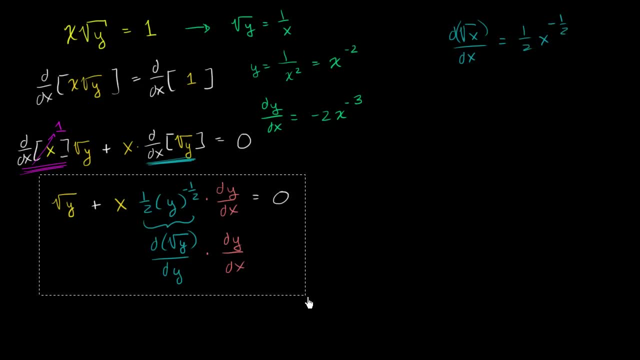 so I have once again more room to work with. So let me cut it actually and then let me paste it. Let me move it over right over here. So we went from there to there. I didn't gain a lot of real estate. 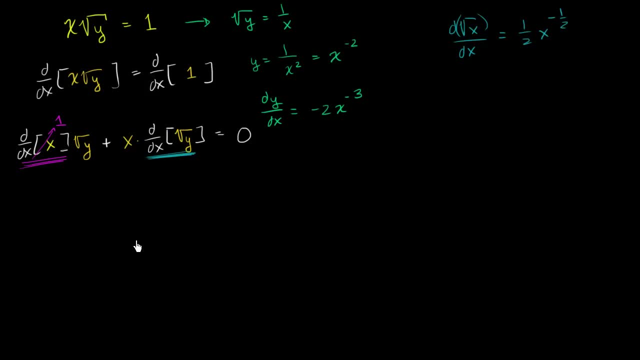 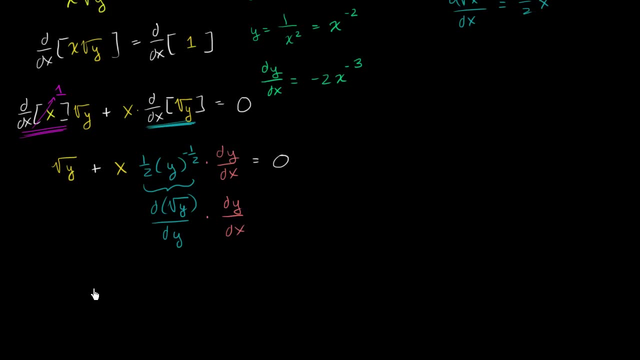 but hopefully this helps a little bit, And actually I don't even like that, Let me put it, let me leave it where it was before. So then, if we subtract the square root of y from both sides, we get, and I'll try to simplify as I go. 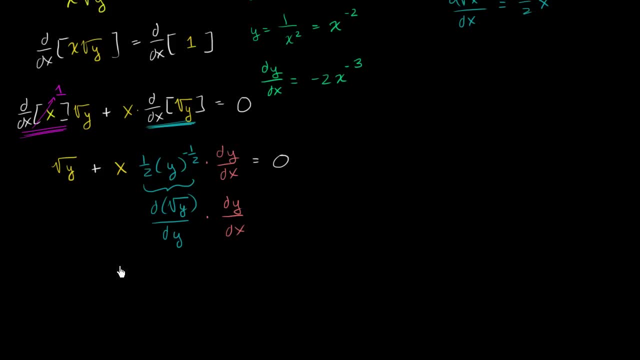 we get this thing which I can rewrite as x times. well, it's just going to be x in the numerator divided by 2 times the square root of y. y to the negative y. 1 half is just the square root of y in the denominator. 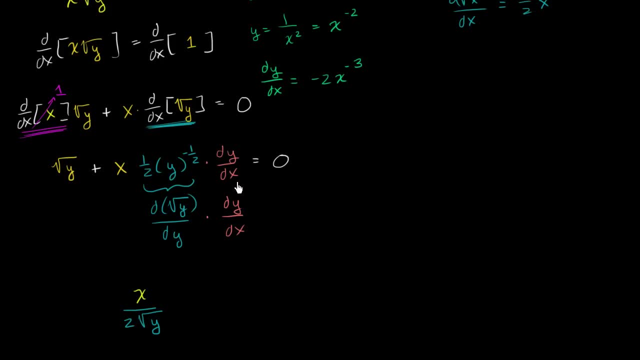 And 1 half. I just put the 2 in the denominator there. times dy, dx, times the derivative of y with respect to x is going to be equal to the negative square root of y. I just subtracted the square root of y from both sides. 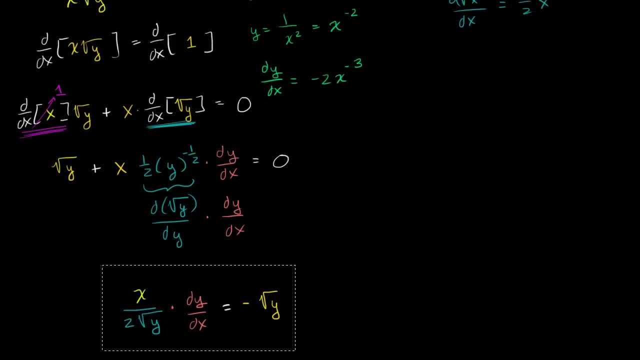 And actually this is something that I might actually want to copy and paste up here. So copy and then paste. So let's go back up here And just to continue our simplification: solving for dy dx. well, to solve for dy dx. 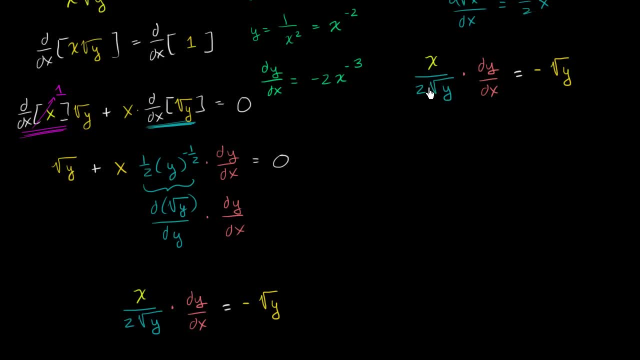 we just have to divide both sides by x over 2 times the square root of y, So we're left with dy. dx is equal to, or. dividing both sides by this is the same thing as multiplying by the reciprocal of this is equal to 2 times. 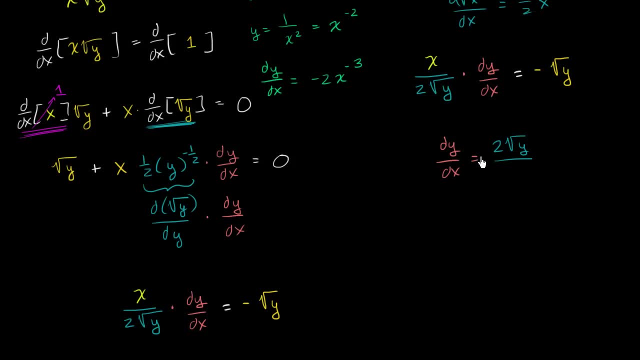 the square root of y over x, x over my yellow, x times the negative square root of y. Well, what's this going to simplify to? This is going to be equal to the square root of y times the square root of y. is just y. 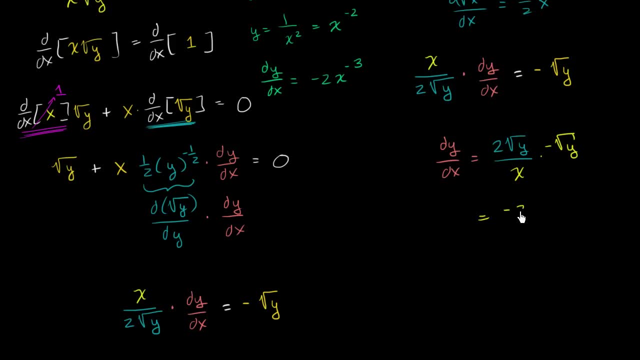 The negative times, the 2, you get negative 2. So you get negative 2y over x is equal to the derivative of y with respect to x. Now you might be saying, look, we just figured out the derivative implicitly. 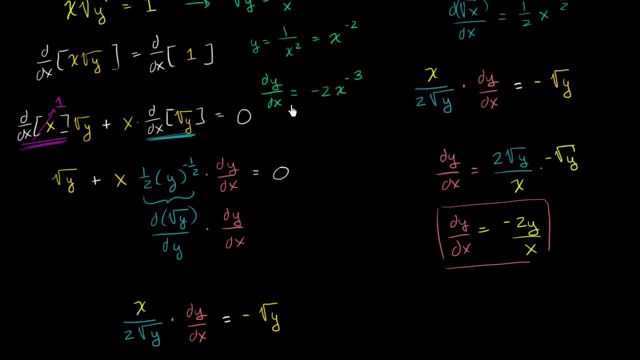 And it looks very different. It looks very different than what we did. It looks very different than what we did right over here When we just used the power rule, we got negative 2x to the negative 3 power. The key here is to realize that this thing right over here,